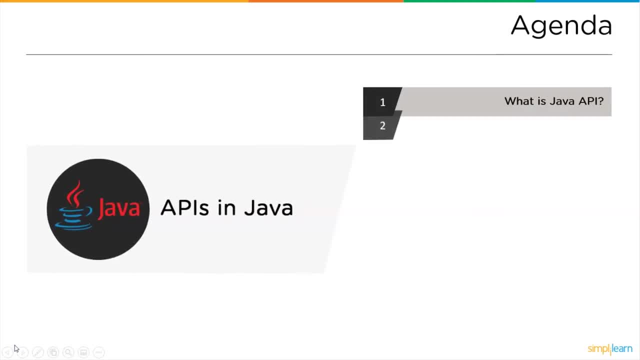 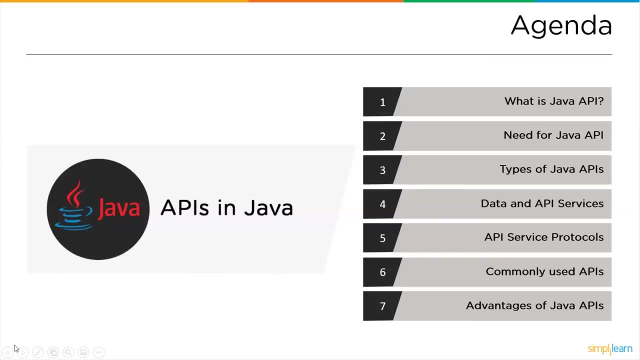 discussion. At first, we will understand what exactly is a Java API and where did it originated from. Followed by that, we will understand the need for Java's API, who exactly uses it and for what purpose. Next, we have the types of Java APIs. Followed by that, we'll understand the data and 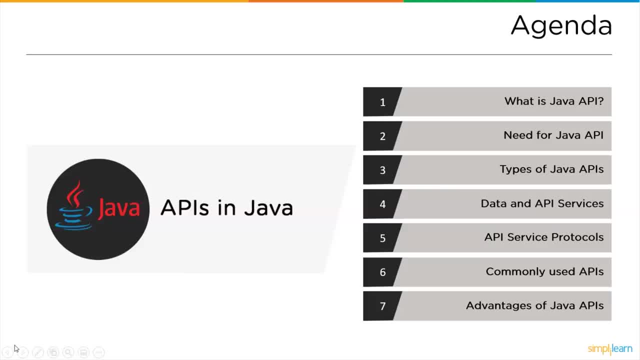 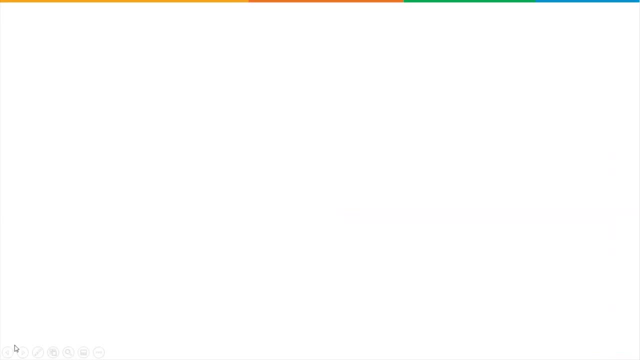 API services provided, then the API service protocols, Followed by that we have the most commonly used APIs list And finally we'll wind up the session by understanding the advantages of Java APIs. So I hope I made myself clear with the agenda. Now let's begin with the first topic. So 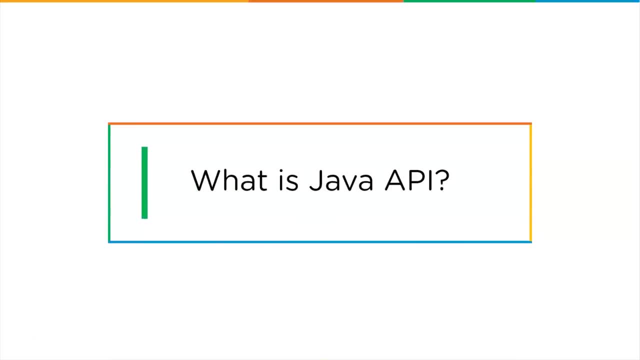 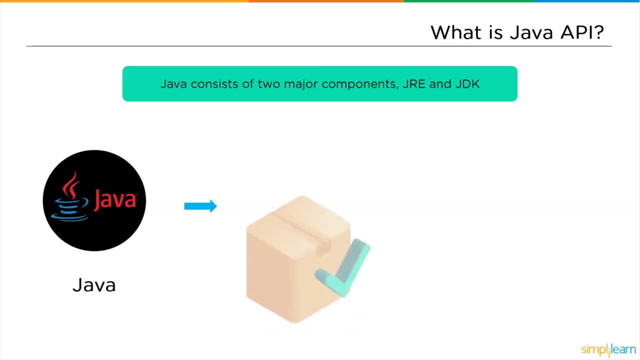 what exactly is a Java API? We will understand what Java is. So basically, Java consists of two major components that are Java runtime environment and Java development kit. So when we get into Java's API we might want to dig a little deep into Java's development kit. So JDK consists of: 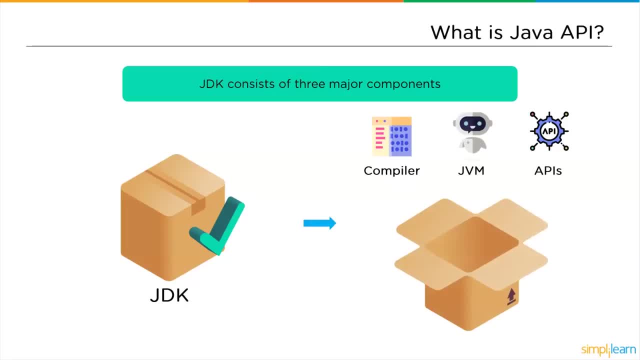 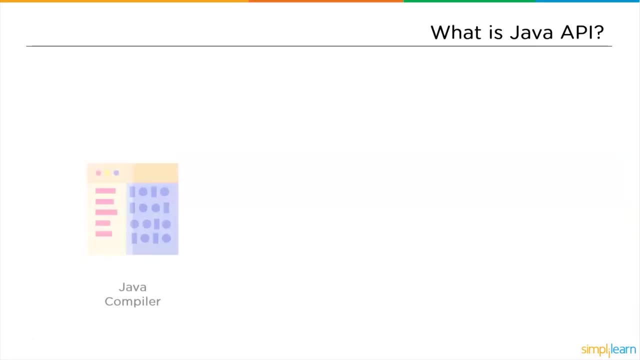 three more major components that are Java runtime environment and Java development kit. So when we look at Java- Java's compiler, Java virtual machine and APIs- Now we will learn each one of them in a bit more detailed way. So at first we have the Java's compiler, So Java compiler can be defined. 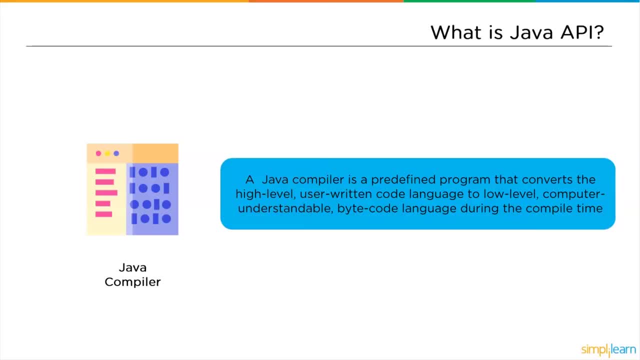 as a software program that is designed to convert the high level, that is, the user return or user readable code, into the computer readable code, that is, the machine level or bytecode. So this particular bytecode will be transferred to the next state where we find the JVM. 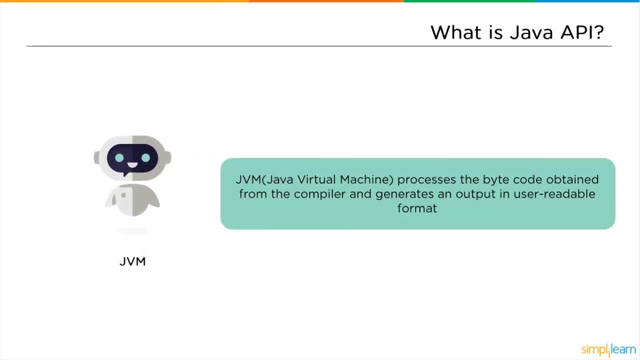 So what is JVM? So JVM is an abbreviation for Java's virtual machine. So Java's virtual machine is responsible for processing all the bytecodes and providing an output to the user. Next we find our topic for today's discussion, that is, the Java API. So just like Java's virtual machine and compiler. 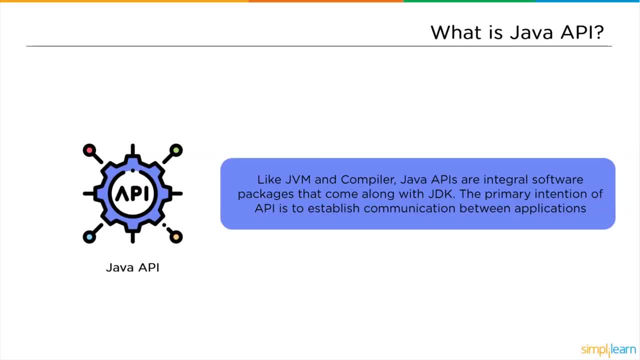 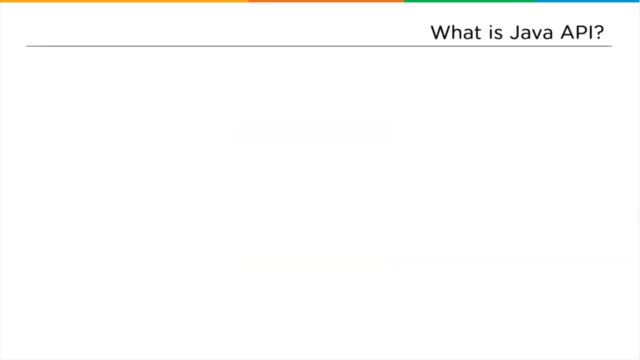 Java's APIs are the integral software packages that come with the JDK. The primary intention of Java's virtual machine is to achieve theЖjjajjajjjajjjaj and JavaScript for the Java API. Java's很多 JVM is a software API, So Java's software app is a JVM. Now Java's JVM is looking at JVM. 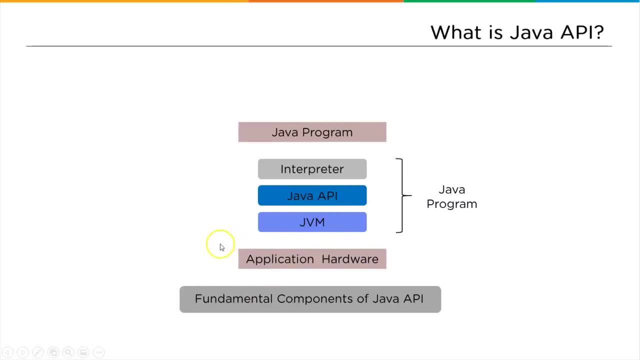 which is the JavaScript API. So Java's JVM's soft JVM is a JavaScript API, So Java's JVM's soft JVM. So Java's JVM's need to be doesn't? we have the application hardware which is responsible for interacting to the Java's program. So this is how the Java APIs architecture looks like Now, followed by this let's dive into. 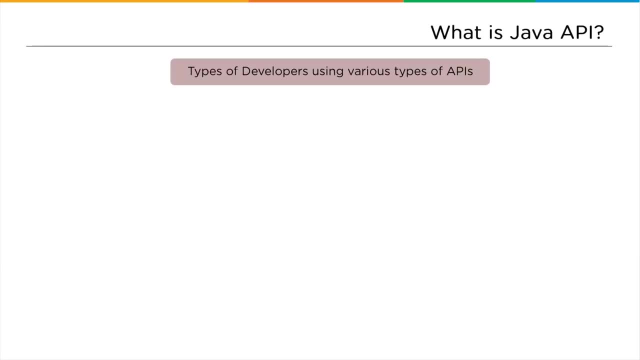 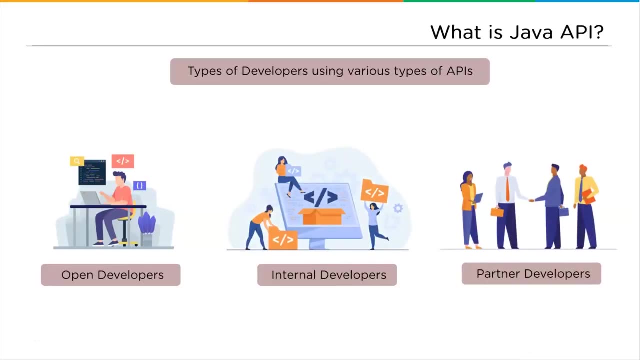 the next topic. So in the next topic we find the types of developers using various types of APIs for different jobs. So at first we have the open developers, next we have the internal developers and at last we have the partner developers. Don't worry, we will understand each of these developers. 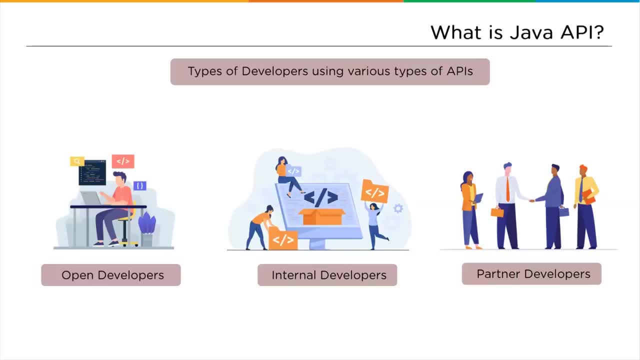 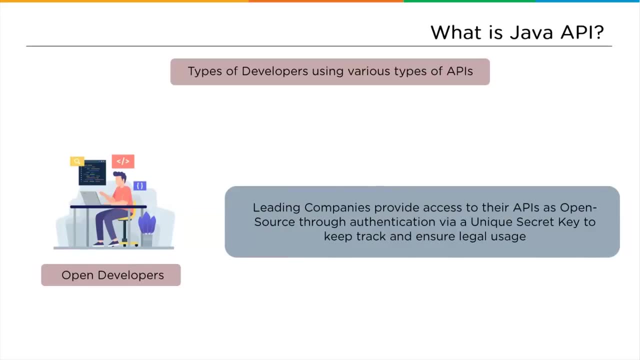 in a bit more detail and along with some examples for a better understanding. So at first we have the open developers. So open developers are used by top-end companies. So leading companies provide access to their APIs as open source through authentication via a unique secret key to keep track and ensure the legal usage. So basically, what happens here is there. 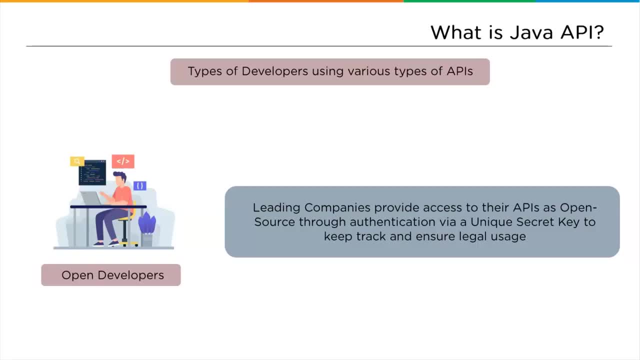 might be some big companies like social media companies or some more other companies which provide the API they use to open up their APIs. So they use the API to open up their APIs So they use for their applications as open source to the developers. So these open developers get. 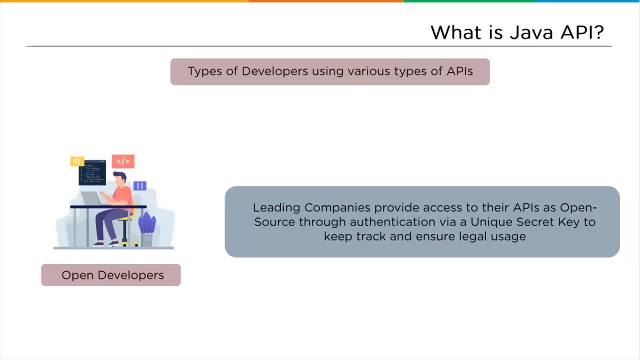 access to their APIs through getting authentication. So they'll be creating a profile, they'll be providing the research details of their application, like what are they using that particular API for and other reasons to use those APIs. Then they get the unique secret key from the 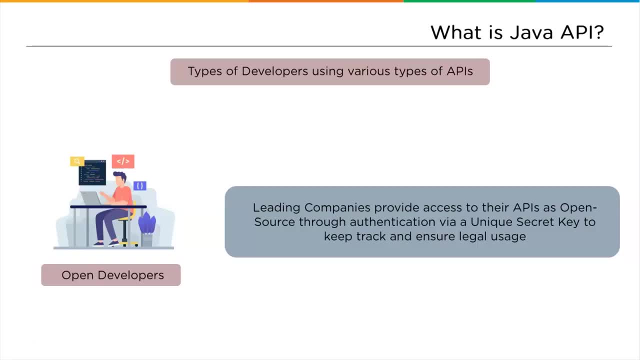 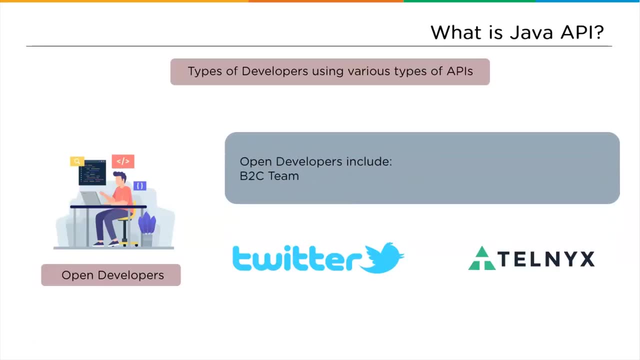 owner of that API, and that's done just to keep track that the API provided is not misused. So the open developers majorly include the B2C teams, and some of the major companies that provide the APIs for open developers are Twitter and Telnyx, So one best example is the Twitter. 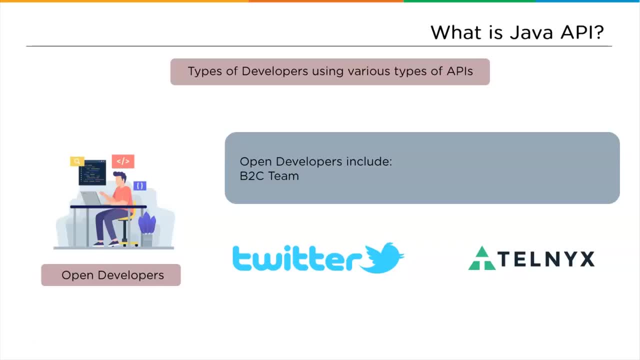 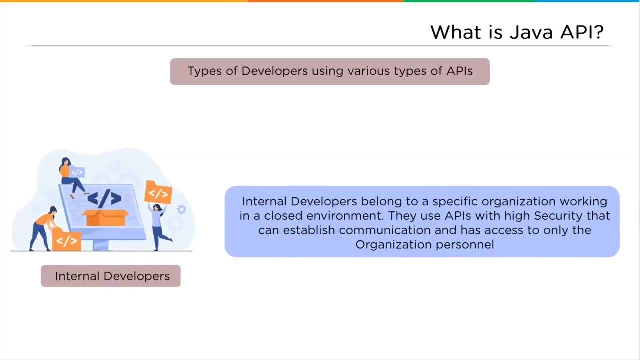 where the Twitter provides Twitter API for the Twitter developer accounts for using that for any kind of developing things or some data science applications and much more. So followed by the open developers. next we have the internal developers. We can consider internal developers as an organization, So the internal developers belong to a specific. 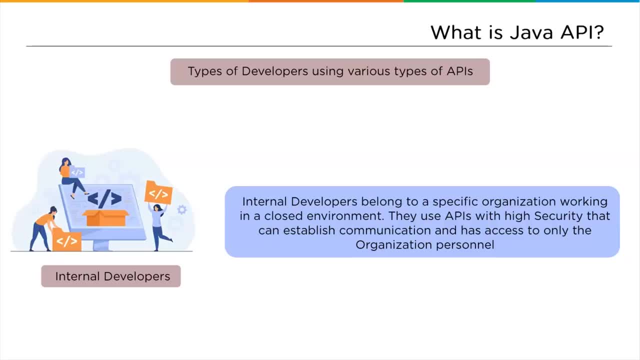 organization and work in a closed environment. These APIs run with a high security that can establish communication between the application and the application hardware. So only the internal developers, that is, the developers belonging to that particular organization, have the access to that particular API. So this particular type of APIs. 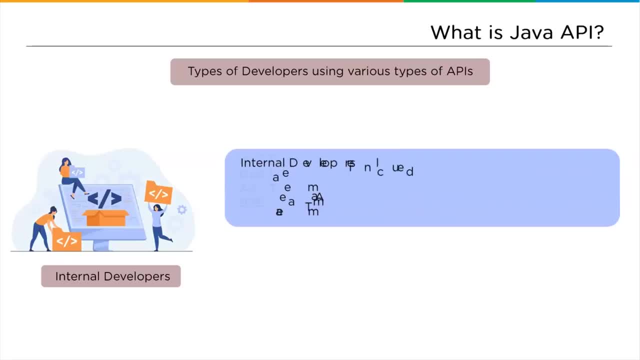 run on a high security level. So internal developers majorly include B2C teams, B2B teams, A2A teams and B2E teams. So some of the major companies that provide the internal APIs are Instagram, Google Mail and Google Cloud. 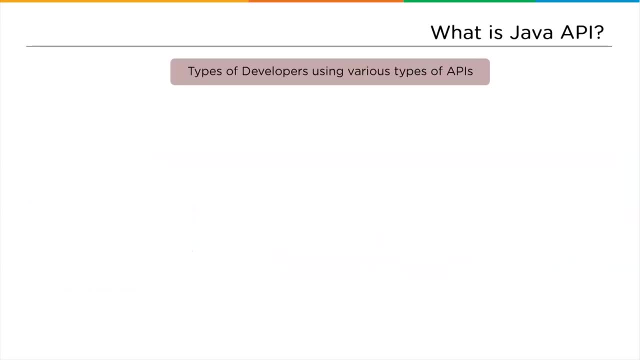 Virtual Machines. Next, we have the partner APIs. So the partner developers are similar or like internal developers, but the only difference is there is a collaboration between two or multiple companies. For example, consider yourself to be linked with a different company and you both wanted to create an application, so only you both can have access to that particular API that you're using to. 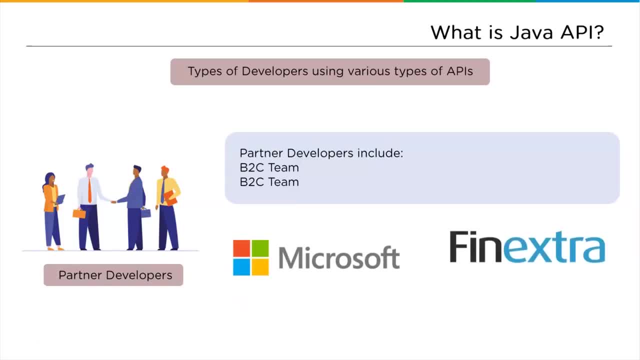 create your application. So partner developers majorly use the B2C teams, and the major companies providing the partner APIs are Microsoft and Finnextra. So with this we finish the first topic. that was what is API and who exactly use it. And so with this we finish the first topic. that was what is API and who exactly use it. 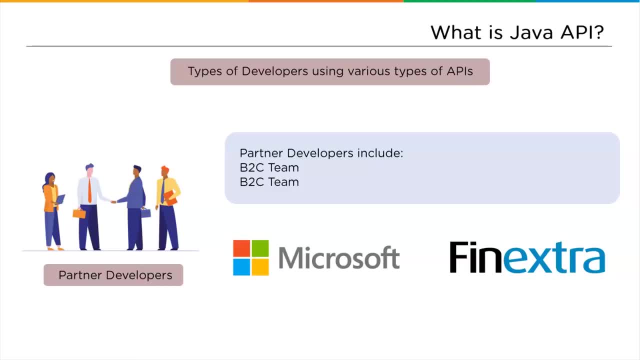 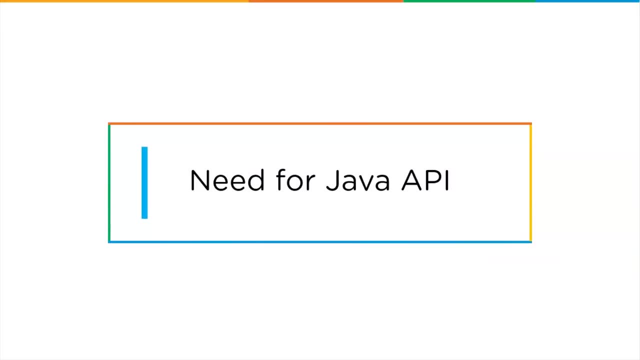 exactly uses it and for what purposes. now we dive into the next segment, where we learn the need for java apis. so why exactly we need java apis now? java apis are used for multiple reasons, but the three most important reasons for which we use java apis are to streamline the operations. 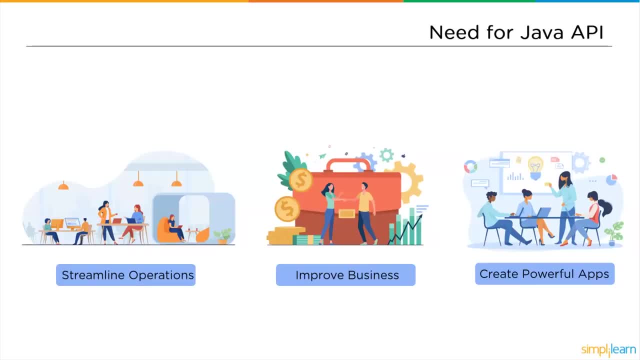 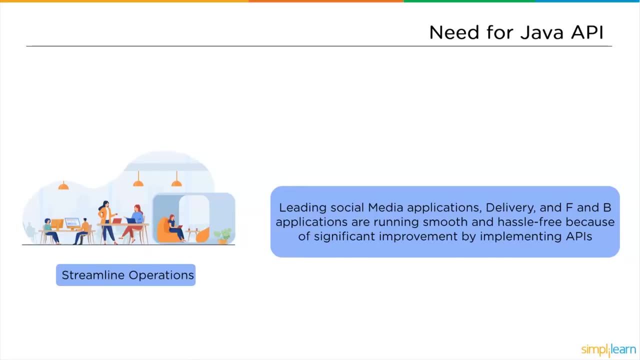 improvise the businesses and finally create some powerful applications. we will discuss each one of them in a bit more detail. so the first one is to streamline operating procedures. we have multiple social media applications like twitter, facebook, whatsapp, etc. followed by that, we have multiple delivery applications, such as amazon, flipkart. then we have the fnb, such as zomato, swiggy, etc. 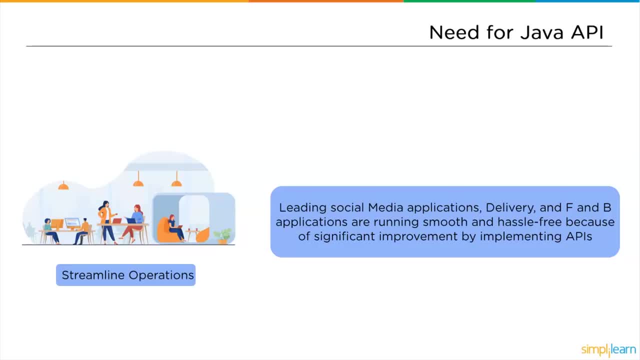 so all these applications are running smooth and hassle-free because of the significant improvement in the implementation of java apis. by using java's apis, users are provided with multiple options on the java apis platform, so they can use java apis to run their java applications on the java apis platform. 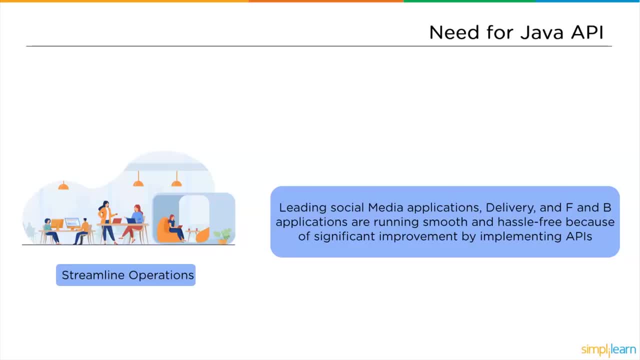 the screen, so this kind of approach makes the functionality very simple and easy to use. followed by this, the next important requirement is to improvise the business. introducing apis to the public leads many companies to release private data to generate new ideas fixing existing bugs and receive new ways to improvise operations. the twitter developer account is an example for 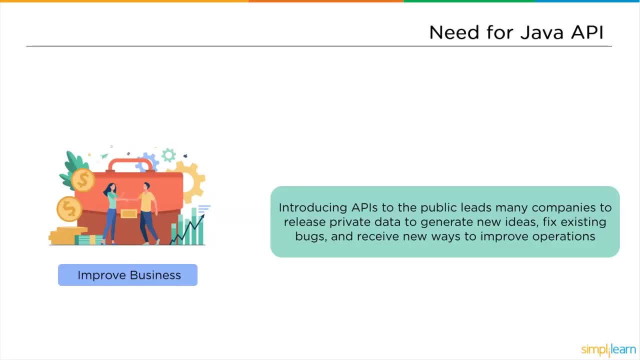 api that gives programmers private api keys to access twitter data and develop applications. followed by that, we have the third one, which is to create the powerful applications. online banking has changed the industry forever, and apis offer the customers ability to manage their finances digitally with complete simplicity, so this is made possible only by the use of apis. 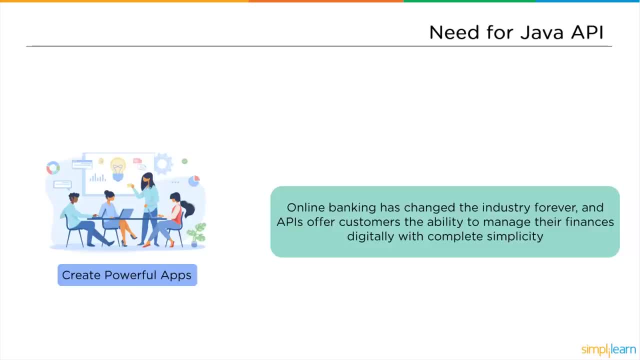 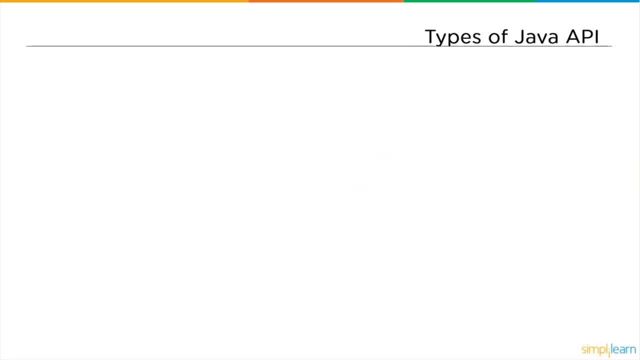 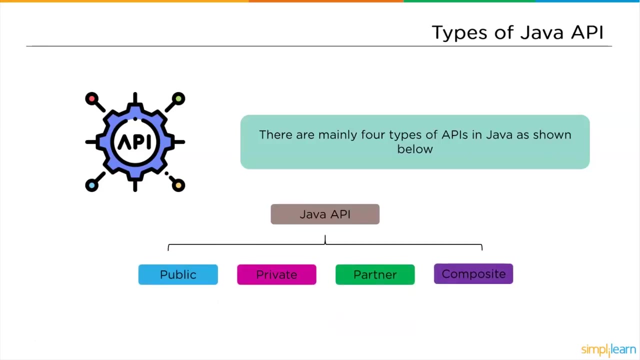 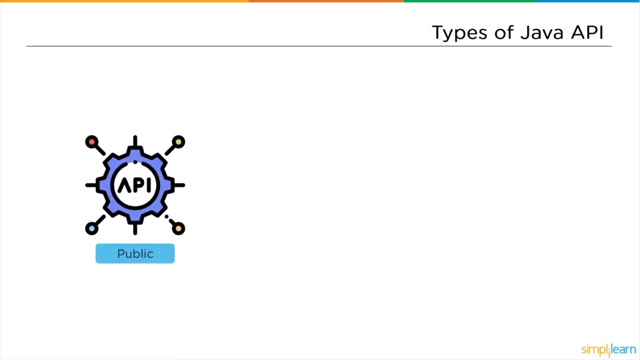 now, followed by this, we will dive into the next topic, where we understand the types of java apis. so basically, there are four different types of apis in java. they are public, private, partner and composite. we will discuss each one of these apis in a bit more detail. at first, we will deal with the public api. so what are public apis? 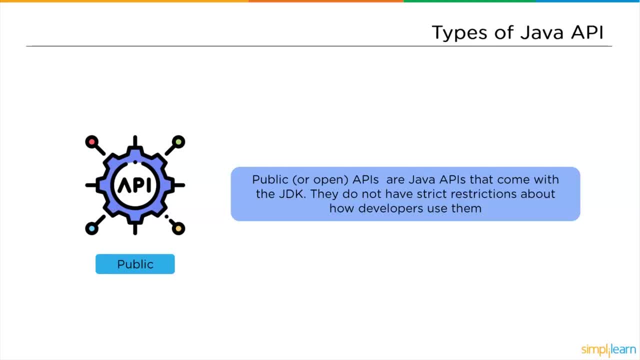 public means open. so public or open apis are java's apis that come with the jdk and they do not have any strict restrictions about how developers use them. so, followed by the public apis, we have the private apis. so the private or internal apis are developed for a specific 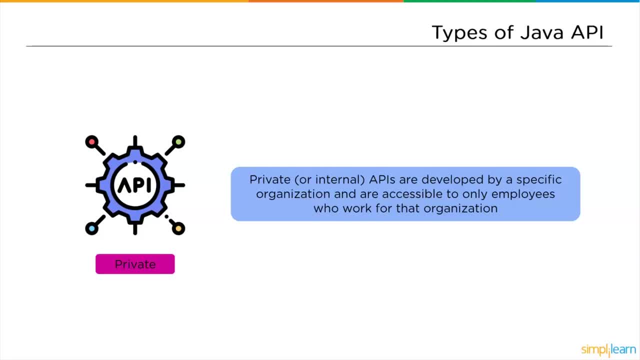 organization, these particular apis will be accessible through the authentication by only the employees belonging to that particular organization. so, followed by private apis, we have the partner apis. so, similar to private apis, even partner apis are having some authentication process to use. so the only difference is here, instead of one api, 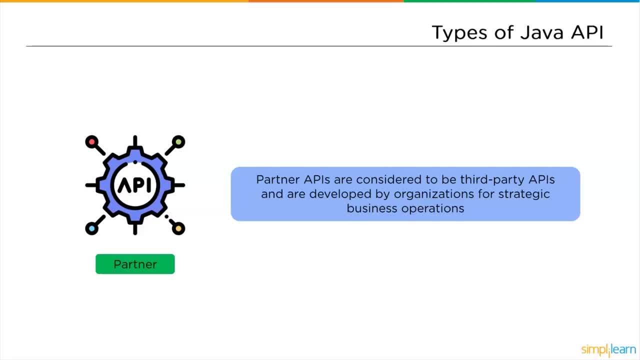 organization. we might have two or multiple organizations, and the employees belonging to that particular group of organizations will be able to access the apis and implement them or use them, followed by partner apis. we have the last one, which is the composite api. composite apis are micro services and developers build them by combining several service apis. now, 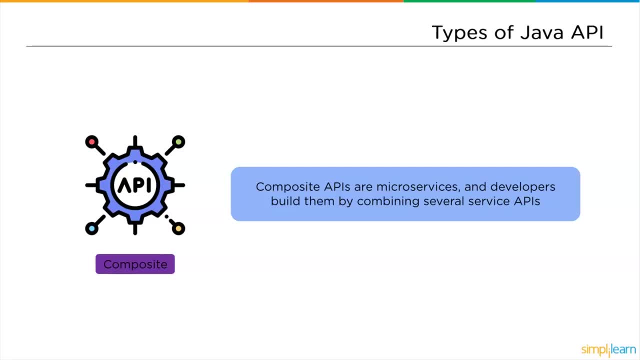 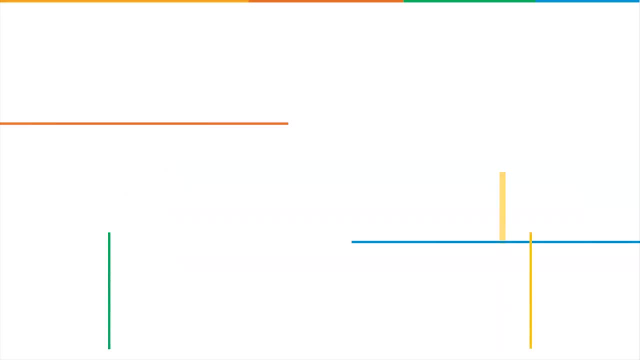 that we have covered the different types of apis, let us now discuss the categorization of java apis based on the services that are being used to create them in java and complex APIs. we will also talk about the types of java apis in the upcoming videos. different varieties of apis in java provide so data, and api services are another way to 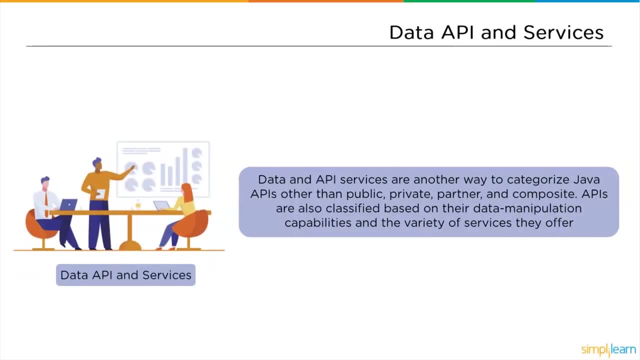 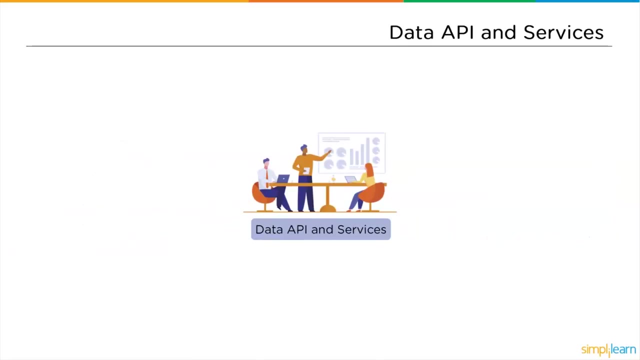 categorize java apis other than the previous type, which is the public, private partner. and composite apis are also classified based on their data manipulation capabilities and the variety of services they offer. so this type of categorization has four different types, which are the internal api services, external api services, crowd operations and user interface services. we will understand. 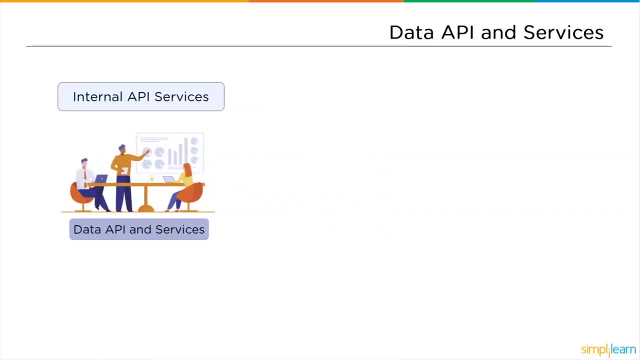 each one of them in a bit more detail. at first, we will understand internal api services. internal api services are developed to offer organizations services specific to that particular organizations. these services include only complex data operations and internal processes, followed by internal api. we have the external api, external api, our 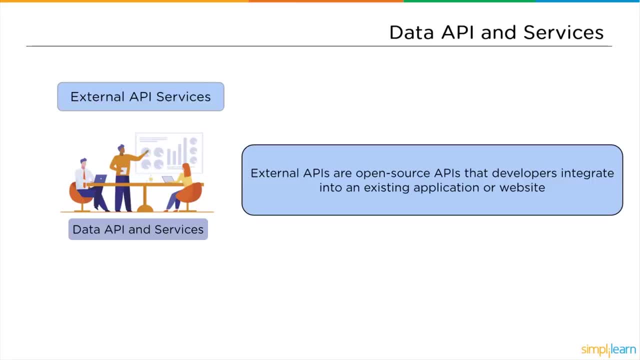 open source APIs that developers integrate into existing application or website. So internal APIs are something similar to private APIs and external APIs are something similar to public APIs. Next we have the CRUD operations. So CRUD APIs provide data manipulation operations over various data storage units, such as software. 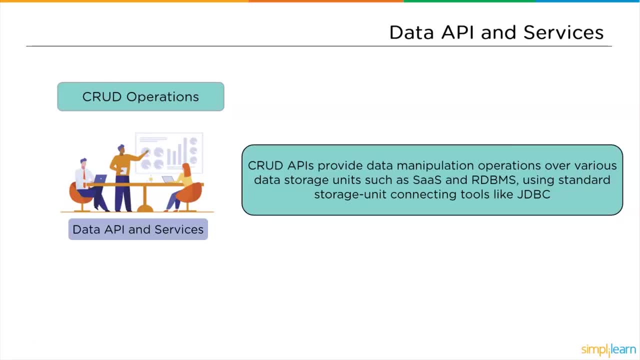 and service- that is, SAS, and relational database management systems, such as RDBMS, using standard data storage unit, connecting tools like database connectivity- that is, JDBC, etc. Next, we have the user interface services. User interface service APIs are open source APIs that allow developers to build user interfaces. 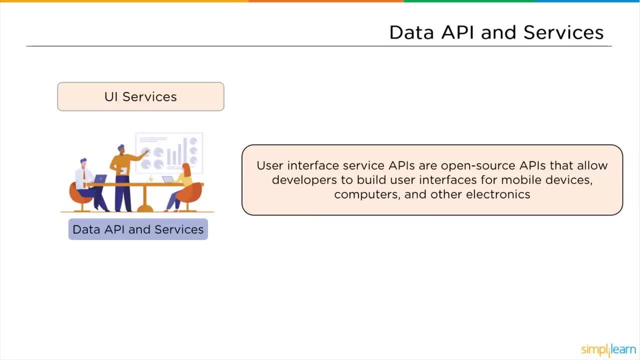 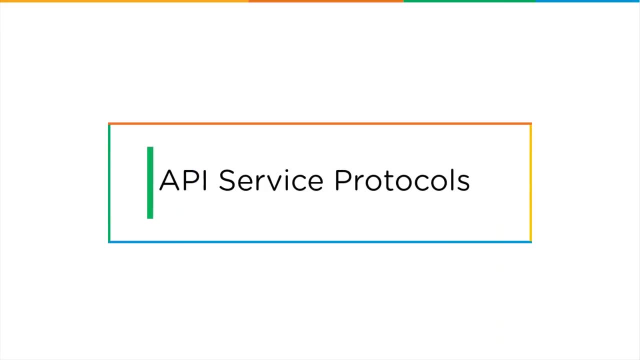 for mobile devices, computers and electronics. Now let's examine the rules and protocols that Java APIs must follow. So that brings us to API service protocols. The rules and protocols guide the different functionalities of Java APIs. So different APIs have different service protocols. 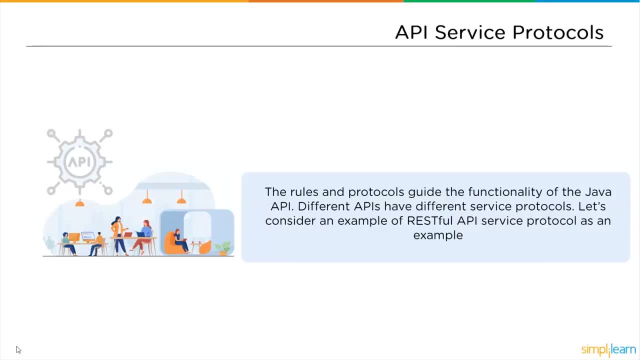 Let's consider an example for RESTful API service protocol as an example. So for a typical RESTful API developers must follow the following rules. For a typical RESTful API, developers must follow these rules: Stateless Uniform Interface, Client Server Cache Layer. 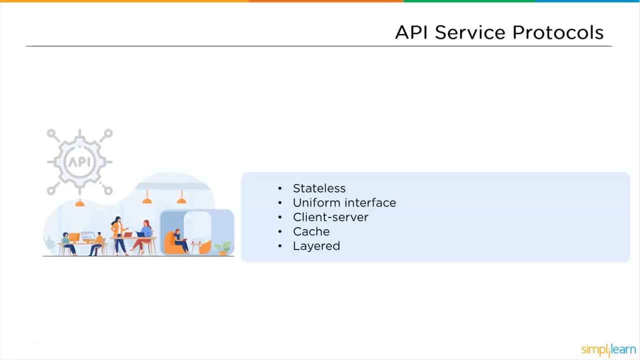 No worries, we will discuss each one of these protocols in detail. First, we will discuss Stable. So what exactly is stateless? So, since the RESTful API follows client-server architecture, by default, it is recommended that RESTful API services to be stateless all the time. 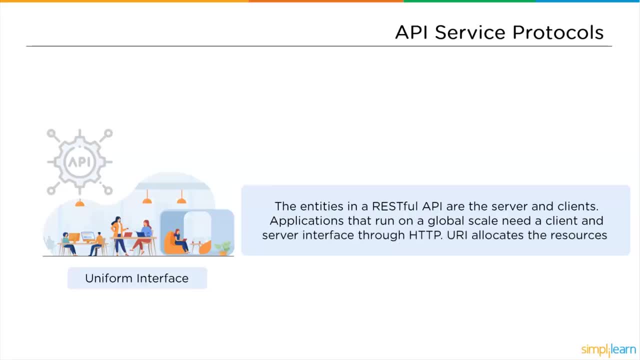 Next we have the Uniform Interface. The entities in a RESTful API are server and clients. Applications that run on global scale need Uniform Client and Server Interface through Hypertext Transfer Protocol or HTTP, and Uniform Resource Identifiers- URI- will allocate the required resources. Next we have the Client-Server. 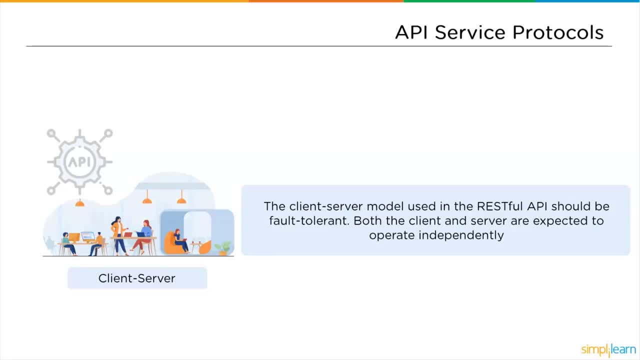 The client-server model used in the RESTful API should be fault tolerant. Both the client and server are expected to operate independently. The changes made at the client end should not affect the server and vice versa. Next we have the Cache. Including a cache memory allows the application to record intermediate responses and run faster. 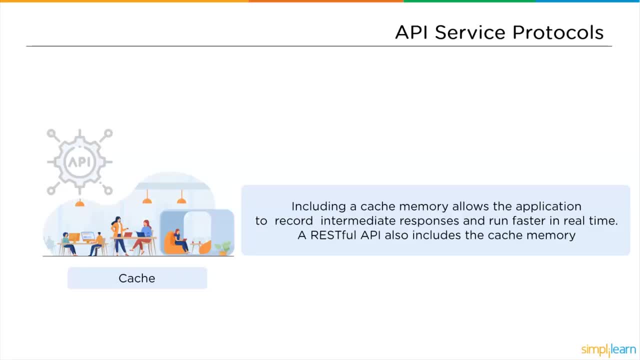 in real time. A RESTful API also includes the cache memory And next we have the Layer. A RESTful API is built using layers. Layers of API are loosely coupled or independent from each other. Each layer contributes a different level of hierarchy and also supports encapsulation. 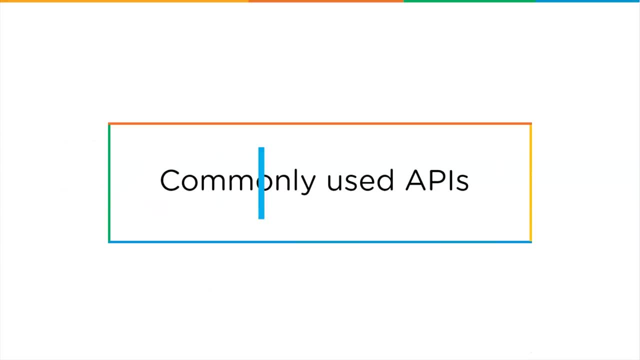 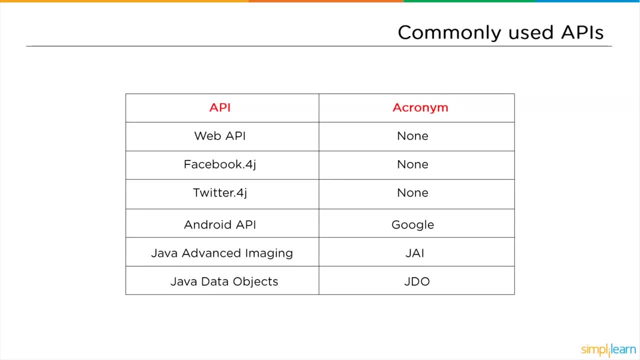 Next we will go through some frequently used APIs. So this is the list of most frequently used APIs in real time. So we have Web API, Facebook 4J, Twitter 4J, Android API, Java Advanced Imaging, Java Data Objects. 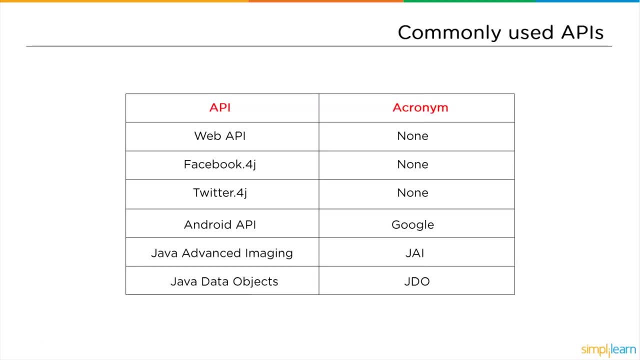 You can also see the acronyms for them in the right column. So some of them have no acronyms and some of them have acronyms. For example, we have Android API as Google, Java Advanced Imaging as JAI Data Objects. 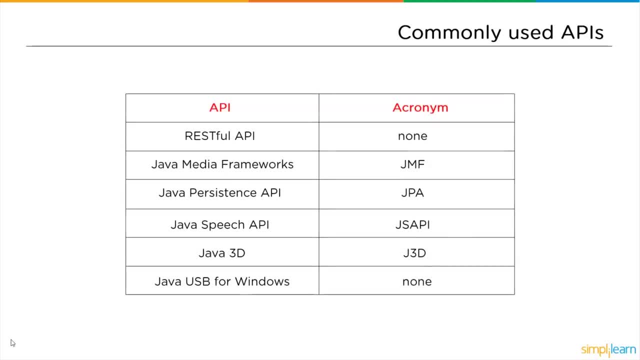 as JDO, etc. So, moving into the next slide, we have a few more APIs, So we have RESTful APIs, Java Media Frameworks, Java Persistent APIs, Java Speech API, Java 3D, Java, USB for Windows, etc. And similarly, on the right column we have their acronyms: 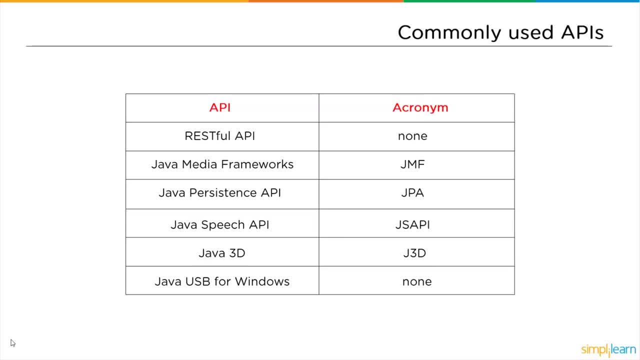 So for Java Media Frameworks, We have JMF. for RESTful APIs, we have nothing. And Java 3D, we have J3D Java Speech API as JS API and few others. So, followed by this, we will advance into the next topic, where we will discuss about the 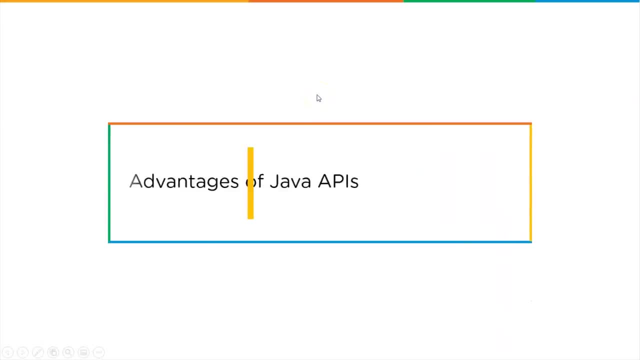 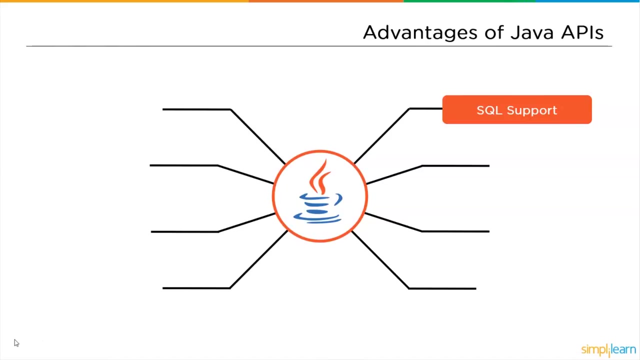 advantages of using Java's APIs. Now, using Java's APIs will help you with multiple advantages. Now we will discuss the most important advantages of using Java's APIs. So the first one, The most important advantage of using Java's APIs, is that they provide extensive SQL support. 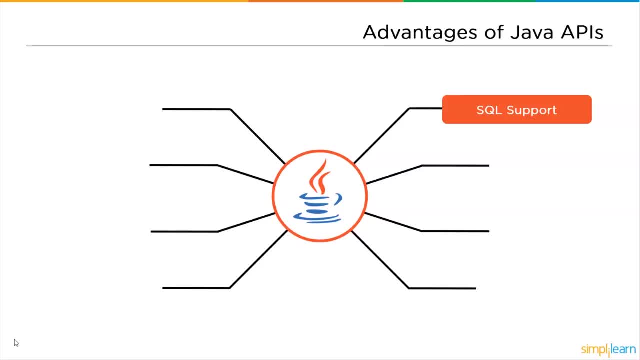 APIs in Java enable a wide range of SQL support services in users applications through a component based interface. Next, we have Applications. APIs in Java provide effortless access to all of an application's major software components and easily deliver services. Next we have Efficiency. Java's APIs are highly efficient because they enable rapid application development. 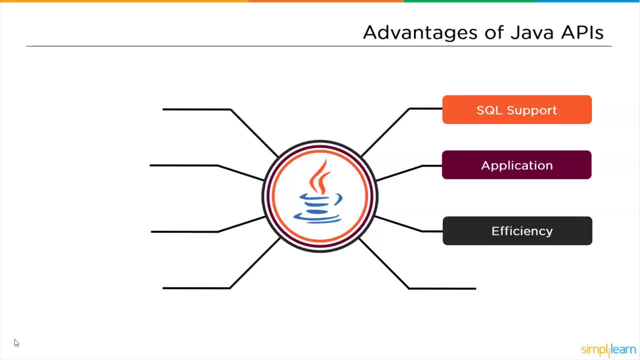 Also, The data that the application generates is always available online. Next, we have the Automation API. allows computers to automatically upload, download, update and delete data automatically without human interaction. Followed by that, we have Integration. Java APIs can integrate to any application and website and provide a fluidic experience.